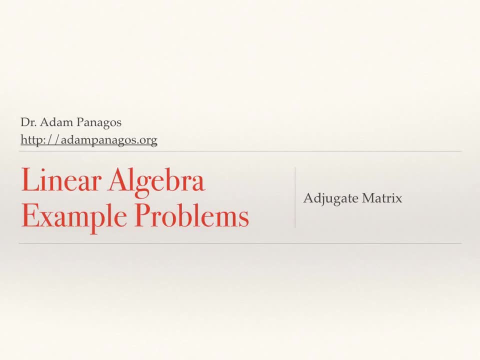 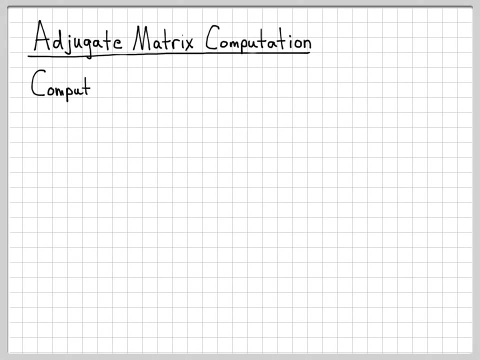 In this example we are going to compute the adjugate matrix of a matrix. So, given a matrix, you can compute its adjugate matrix. So the matrix we're going to work with is the matrix A, which is a minus 2, 5, 1, 4, 1, 0, and a 3, 5, 5.. So that's the matrix A, And what? 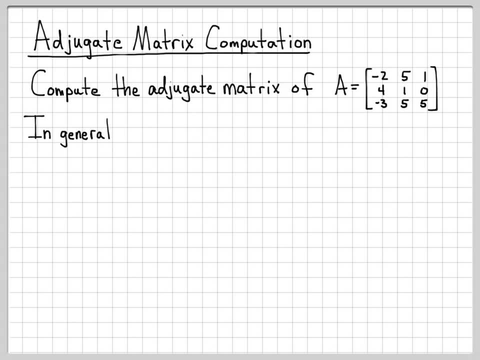 we're asked to do is to compute the adjugate matrix of the matrix A. So first let's talk about the general definition of an adjugate matrix In general when we're working with a square matrix, so again, this has to be for a square matrix, the adjugate of the matrix. 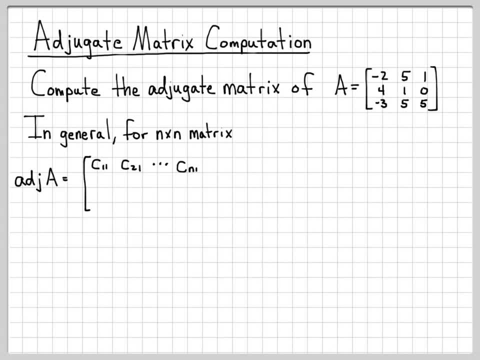 A can be written in this general form: c11, c21,, all the way to cn1,, c12, c22,, all the way down to cn2, and then down this column. So this is what the adjugate matrix form looks. 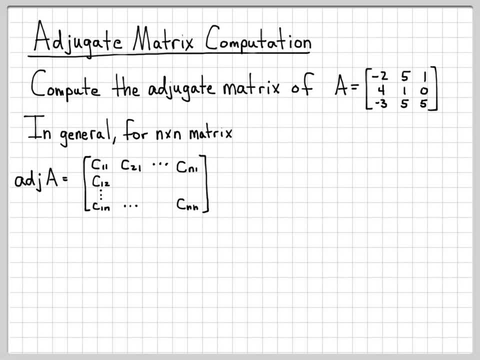 like in general, is just a number, C21 is just a number, C12 is just a number. These are all just scalar numbers And these numbers are actually the cofactors of the matrix A. For our particular problem, since we're working with a matrix A that has n equal to 3, we 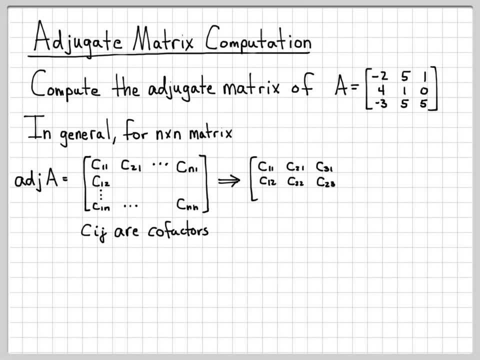 don't have to go to n here, We only have to go to 3.. So if we want to fill this definition, which is a general definition, for our specific case, it turns into this 3 by 3 matrix that we're actually looking to compute in this problem. So there's actually nine numbers. 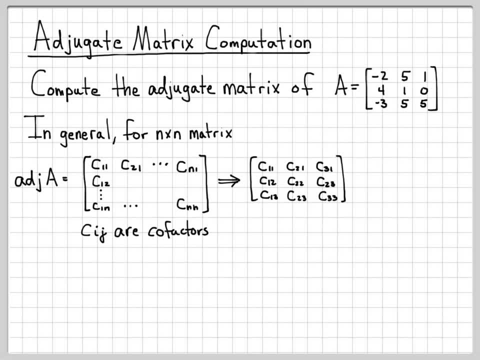 here that I need to know to be able to write down the adjugate matrix. Notice one thing here: The subscripts written here are correct: C11,, C21,, C31, et cetera. across that first row. It looks a little backwards, right. Normally we do rows and columns, So 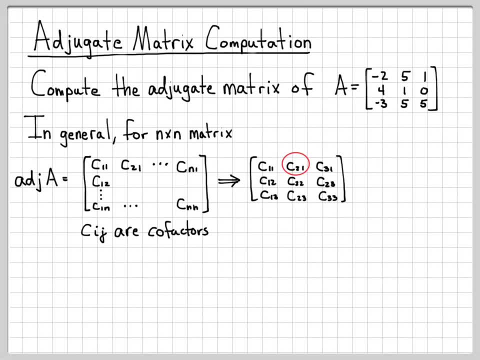 you might have guessed that that should have been C12.. And this should have been C13, because these are in the first row. But the adjugate matrix is actually transitive Transpose in this definition in terms of the cofactors, So this is written down correctly. 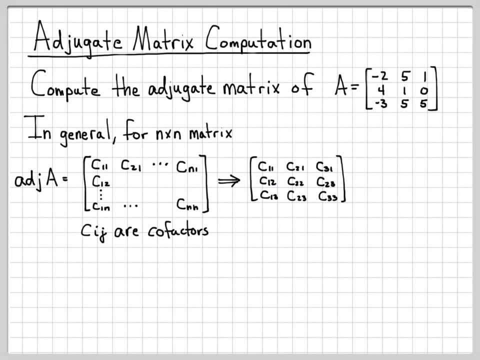 And just be careful when you populate your matrix not to get things out of order. So what do we need to do to actually compute the adjugate matrix? for our particular example, we're working, We need to compute these nine numbers, So let's go about computing those. 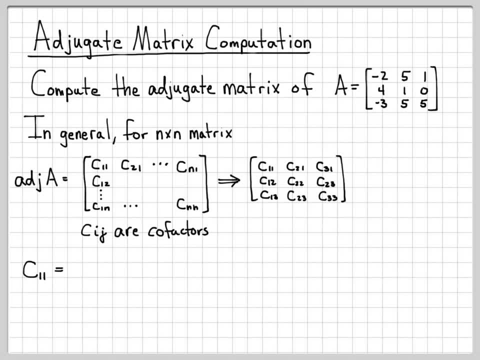 cofactors. So C11 I can get by blanking out the first row and the first column of matrix A. What I'm left with is the 2 by 3 matrix, 2 by 2 matrix 1,, 0,, 5,, 5.. And I can compute the determinant of that And I get the number. 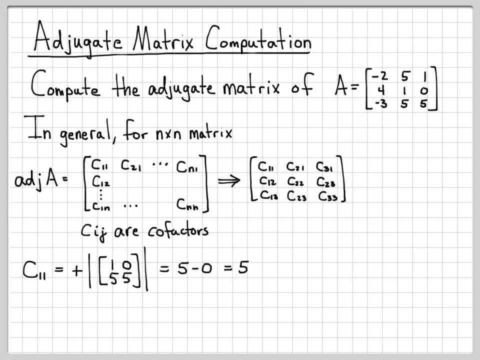 5.. So C11 is equal to 5.. What about C21?? Or C12,, I'm sorry, C12, very similar thing. I need to cross out the first row, second column, And then what am I left with? 4, 0, negative 3, 5.. The other tricky. 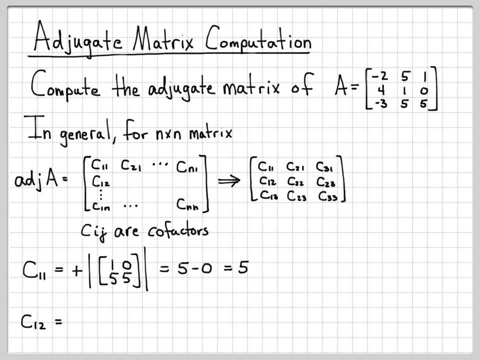 part is remember: when we do cofactors, the sine toggles back and forth. So I'm actually going to have a negative sign here, And then the matrix 4, 0, a negative 3, 5,. like I said, 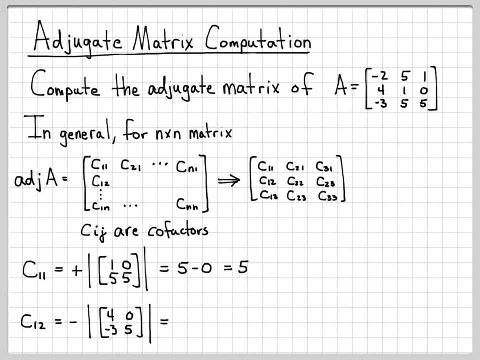 So I need to take the negative of this determinant quantity, So that's the negative of 20 minus 0, which is a negative 20.. And then we can just keep going. We need to compute C13,, et cetera. 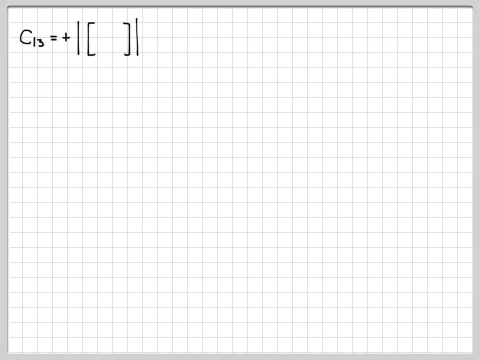 Let's just keep going. C13 is going to be positive. the determinant of some 2 by 2 matrix: 2.. No, So what that 2 by 2 matrix is. I went ahead and wrote down the A matrix again, So row. 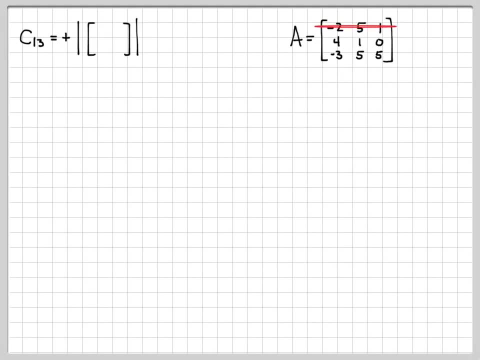 1, sorry, row 1,, column 3, I'm going to strike out. So what am I left with? I'm left with this 2 by 2 matrix. That's the 2 by 2 matrix I need to fill in here. So that's what I've. 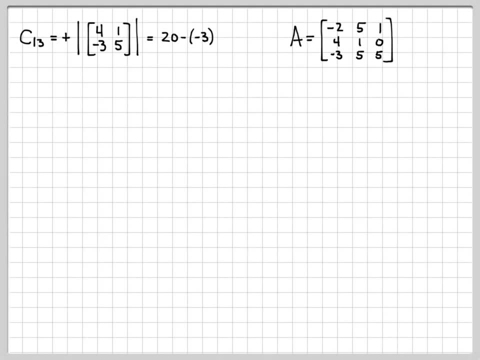 written down right there. I do my little computation: I get 20 minus a negative 3, which is 23.. And we just keep going. C21, it's going to change signs, So it's a negative. I get the. 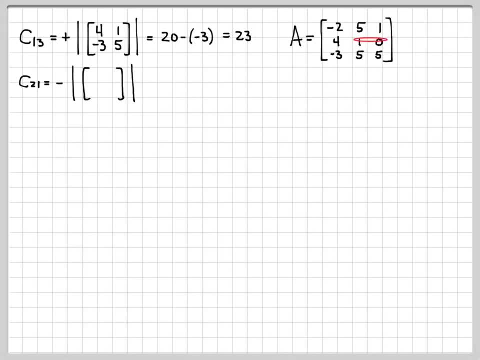 2 by 2 matrix, by crossing out the second row, first column, And I'm left with 5, 1,, 5, 5.. So that's what goes right. there I get a negative 25 minus 5, which is a negative 20.. C22 will.